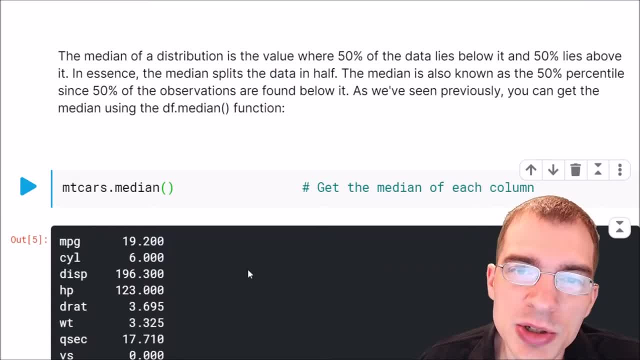 median tell us something similar. They're both measures of what could be considered a central or typical value in a distribution And, depending on how your data is distributed, they could be very similar or even the same, But if you have data with some skewness in it, they can also be fairly different. 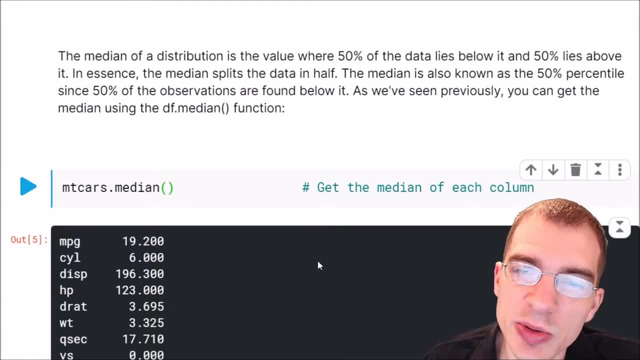 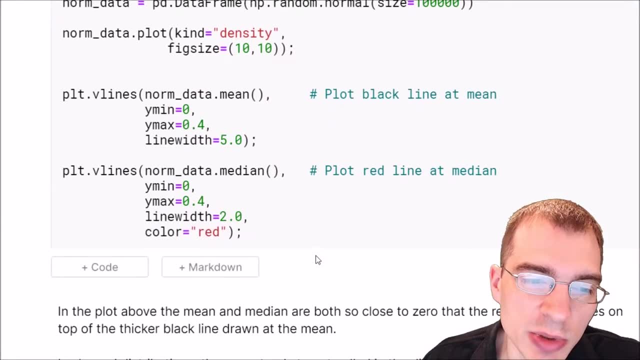 So we'll show a couple of different distributions and the difference between the means and medians to give an example of this distinction. So first we're going to generate some normally distributed data and then we're just going to plot it with the mean and median plotted. 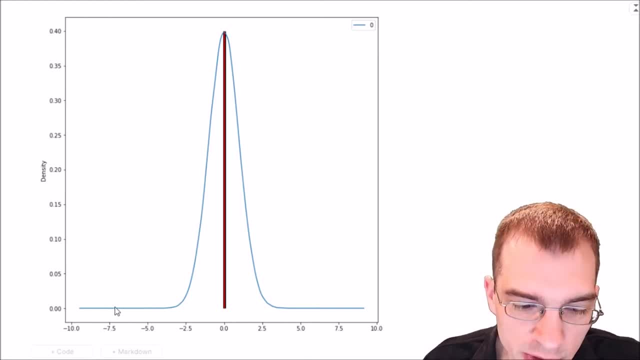 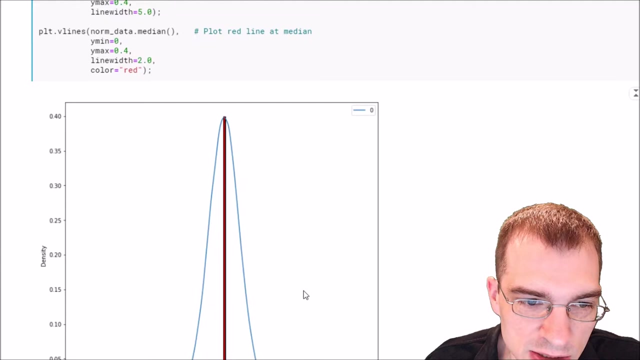 as well. So in the resulting plot of the normally distributed data here the mean and median are exactly overlapped. The median is this red line and the mean is actually a black line that's right under where the median is. So it's hard to even see it because they're 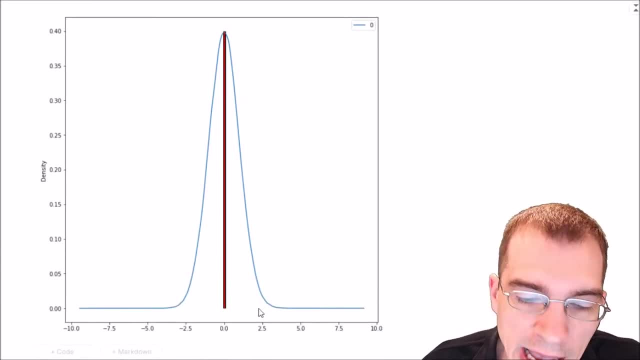 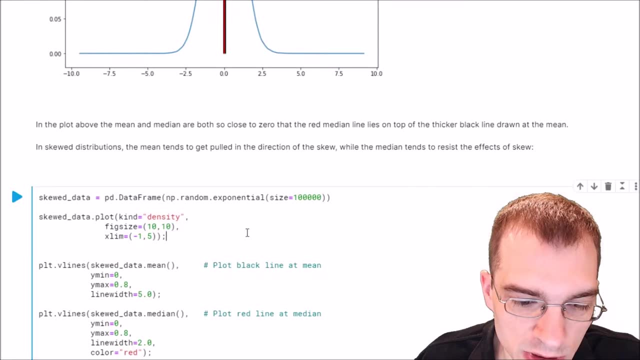 overlapping, But with normally distributed data, the average and the median are in exactly the same place. Now let's try this same thing with some skewed data and see what the difference is. So I'm going to run this and we're going to generate another plot, just with different data And 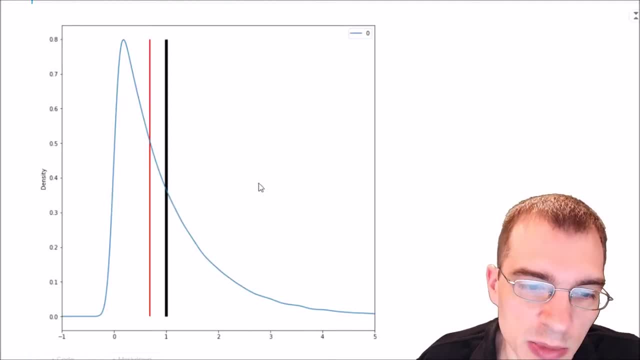 in this plot. here we can see the difference between the median and the skewed data. So the median and the median- The mean bar, the black bar, has been pulled out further to the right by this skewed long tail, whereas the median bar, the red bar, is not pulled. 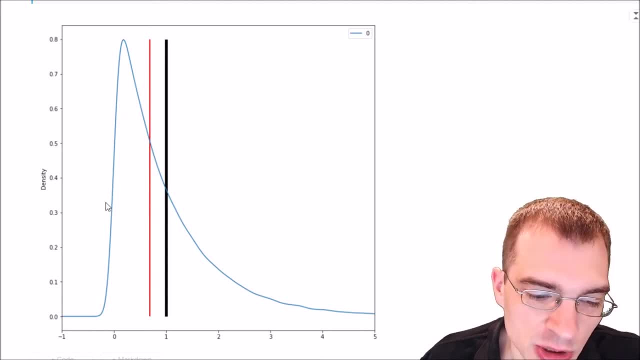 so far to the right. So it has managed to stay closer to the bulk of the data here, because it's not as affected by these more extreme values. We'll give one more example here of a distribution that has some outliers to show that the mean 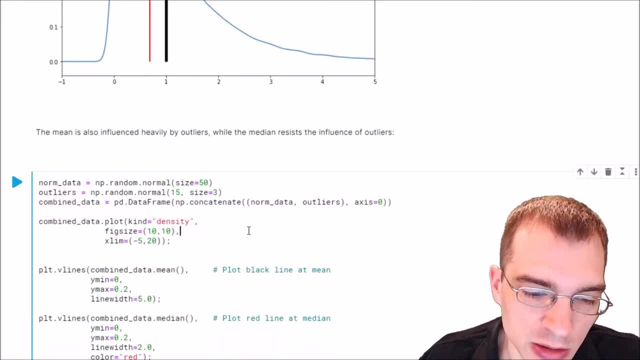 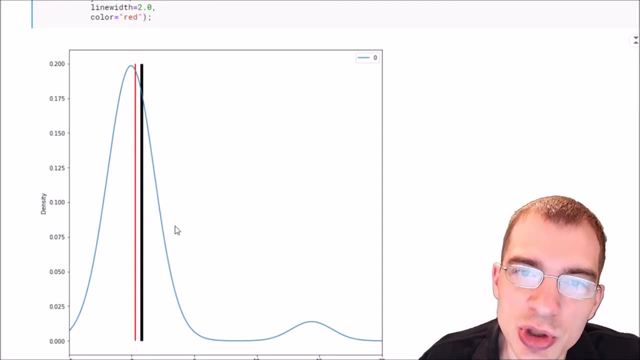 is also affected more by outliers than the median. So we're going to run this. We're going to run this plot now, And we can see here that we have kind of a bimodal distribution where most of the data is right here, but there's also this blip of more extreme. 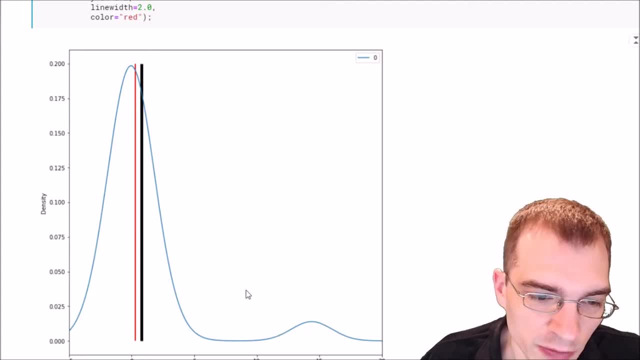 values or outliers up here And for the median. the median is still almost right in the center of this first normally distributed section, whereas the mean, the black bar, has been pulled up more by these outlier values here. Now, since the median tends to be the center of the distribution, the median tends to be 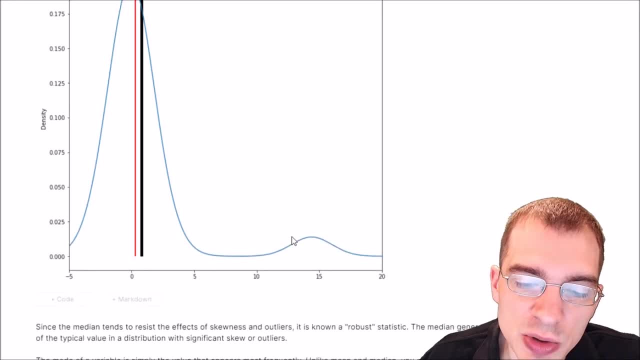 the center of the distribution. So the median tends to resist the influence of skewness and outliers. It is known as a more robust statistic than the average or mean, which is greatly affected by skewness and outliers. So when you're dealing with a distribution that has skewness or outliers, the median 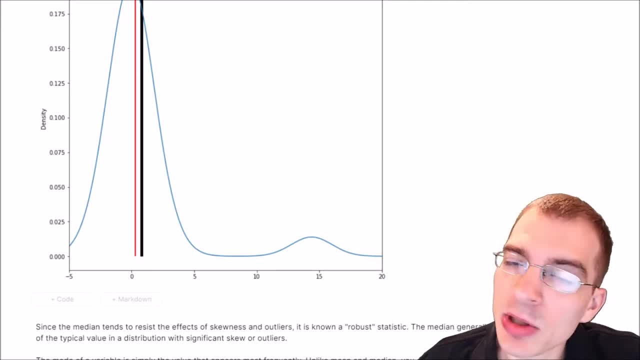 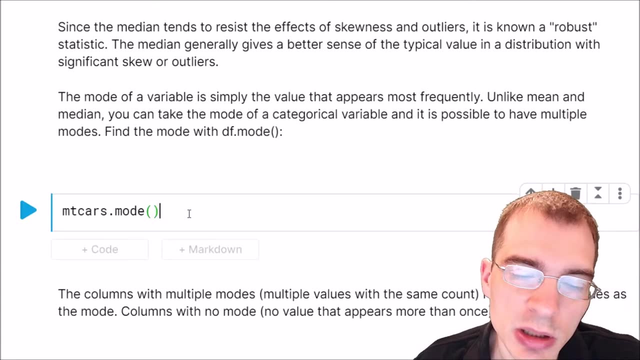 will usually give you a better sense of a typical value than the mean does. Finally, the mode is just the value that occurs most frequently In a distribution or of a categorical variable, And to find the mode you just use mode. So here we can do mtcarsmode. That will get us the most frequent value for each column. 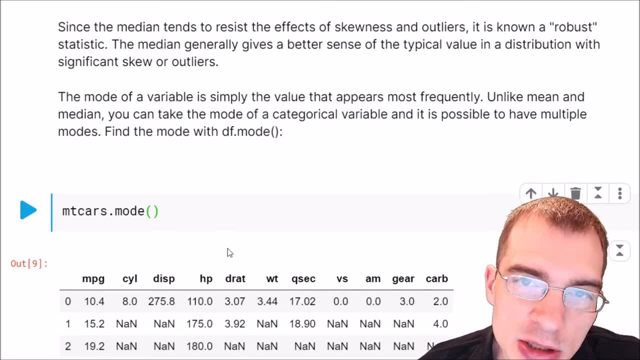 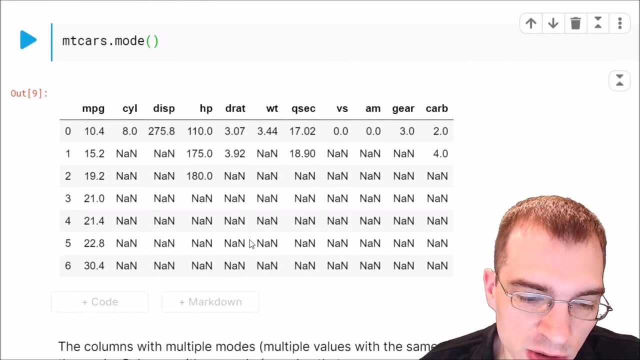 And if you have certain values that are ties, so certain values occur the same number of times and that's the most- then you will get multiple rows returned here. So we can see in the result for mpg for instance, there's probably not that many cars that have the 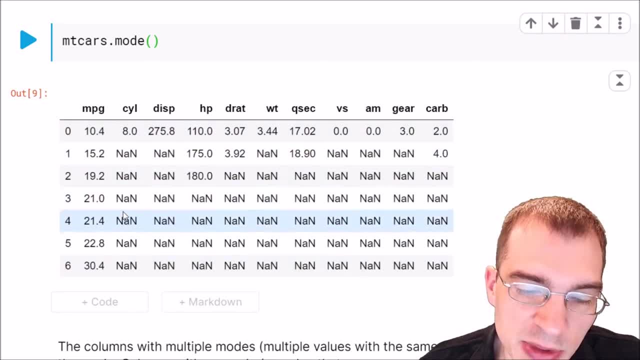 exact same mpgs. So we see six modes listed because maybe two cars have this, two cars have this, etc. So that's why there are six modes listed for mpg, But other things that occur with more frequency, like eight cylinder cars, only have one mode listed. 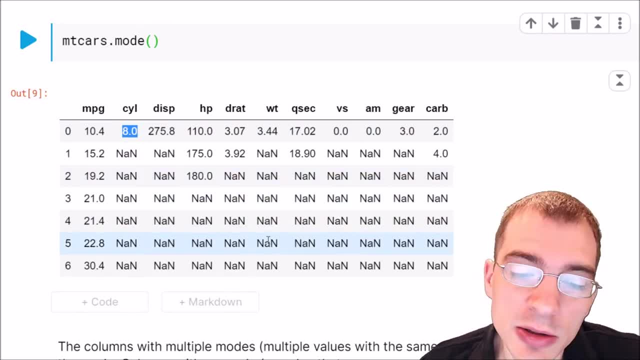 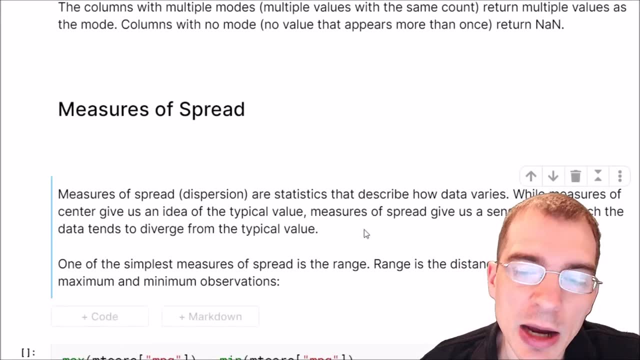 So measures of center give us an idea of the typical values a variable takes on. Measures of spread or dispersion are statistics that describe how data varies. Measures of spread tell us the data tends to diverge from the typical value. Now, one of the simplest measures of spread is just 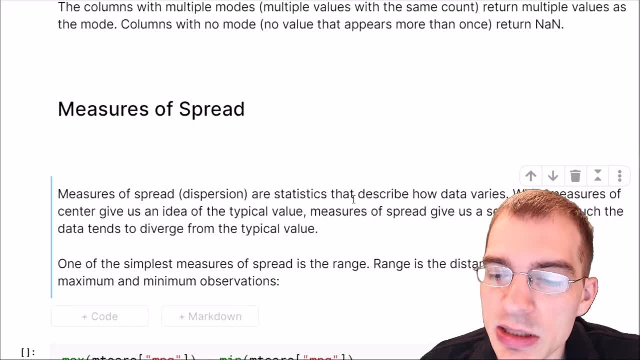 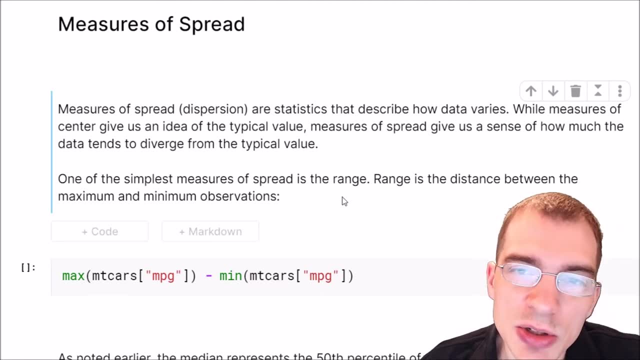 the range of the data. The range is the distance between the minimum and maximum value. So to get that for observations in pandas you can just take the max of a column and subtract the min of a column. that will give you the range. So for the mpg column, for instance, we could say max of that. 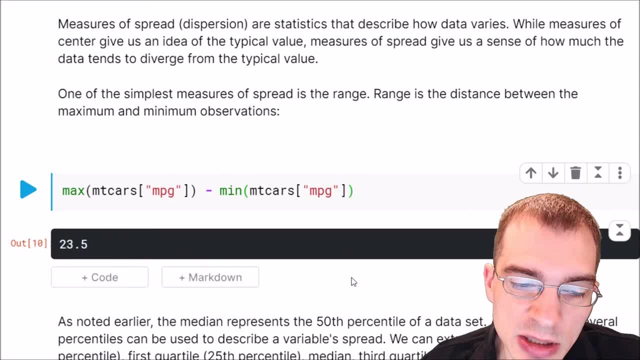 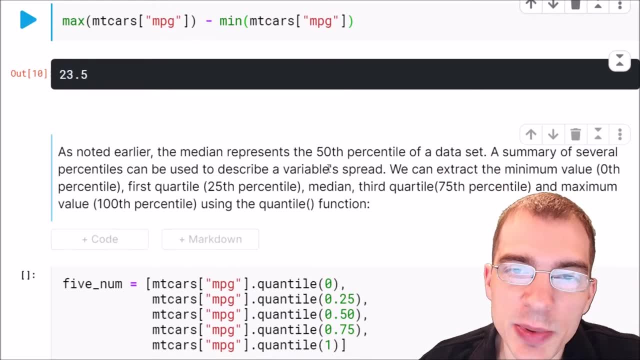 column minus min of that column and we run that and we can see that the range is 23.5 miles per gallon. Now, as we noted earlier, the median of a data set represents the 50th percentile of the data, which means 50 percent of the data is below it and 50 percent is above it. A summary of several 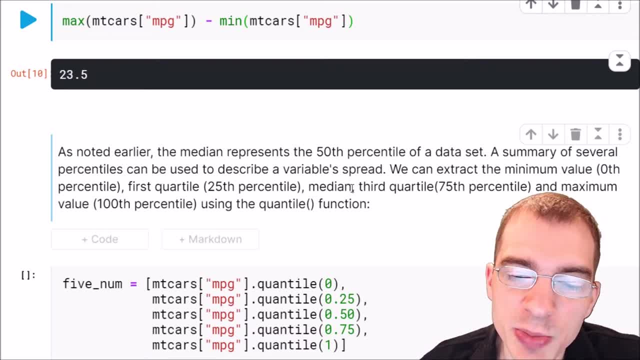 percentiles can be used to describe a variable spread. So one way we can look at the spread of a variable is checking the minimum value, which is the same as the zero percentile. the 25th percentile, which is the first quartile, the median, the 75th percentile. 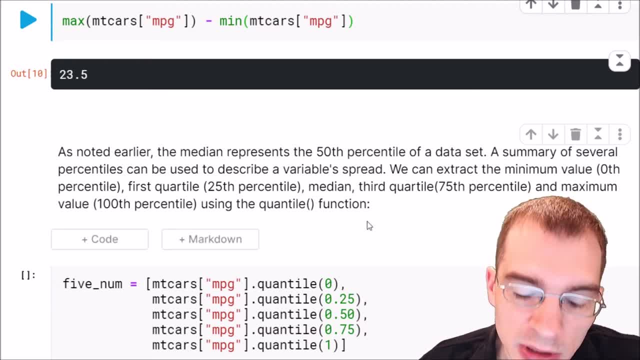 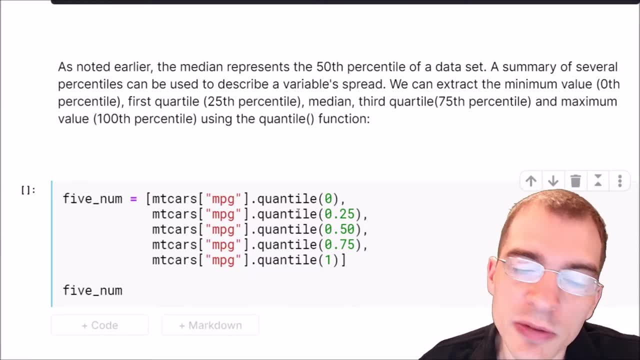 which is the third quartile and the maximum, And we can check quantiles, which means a given percentile in pandas, using the dot quantile function. So to extract this so-called five number summary, we can just take our mpg column, run dot quantile and then enter the value for 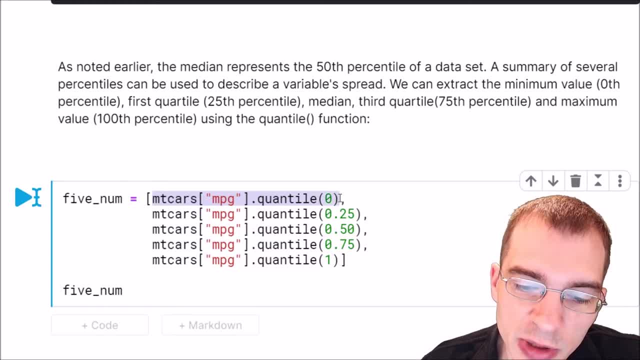 each of the quantiles we want to get. In this case, we're going to use the dot quantile function to say zero for the minimum, 0.25,, 0.5, 0.75, and 1 for the maximum, And we run this. we're going to 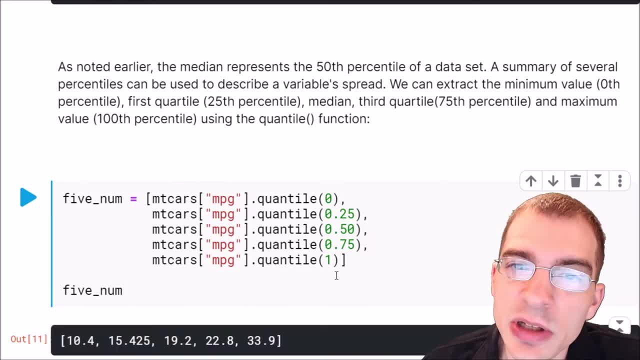 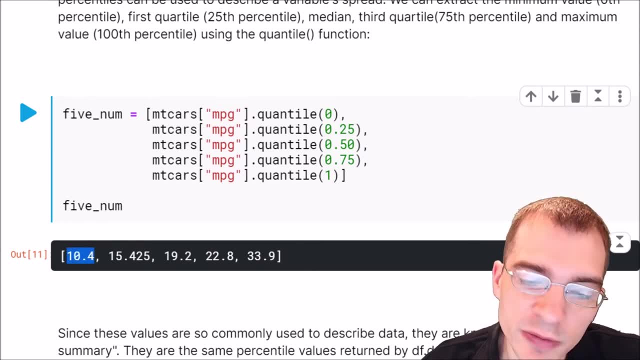 make a list of five numbers that's going to give us a sense of the overall distribution of this mpg variable. So you can see here in our five number summary, the minimum is 10.4 mpg, the max is 33.9,. we see the median and then we get some intermediate values here. that are the quartiles. 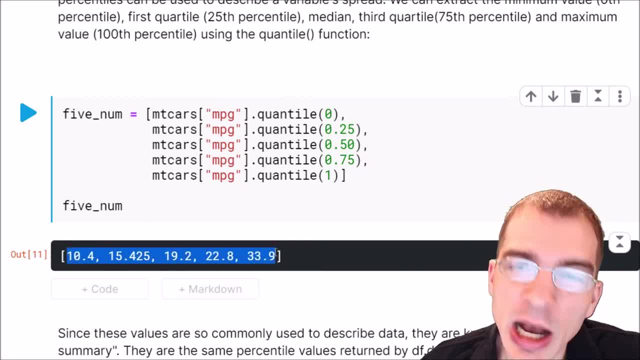 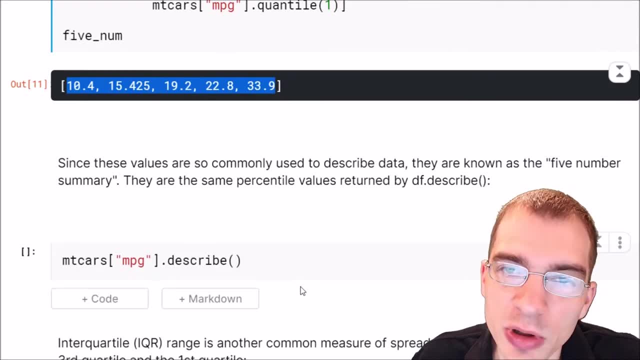 Since these five number summary values are so commonly used, you can actually use the quantile function to get the quantile value. So we're going to actually get them automatically using the dot describe function in pandas we've learned about before. So we could have just taken the column and run dot describe on it and that's going to. 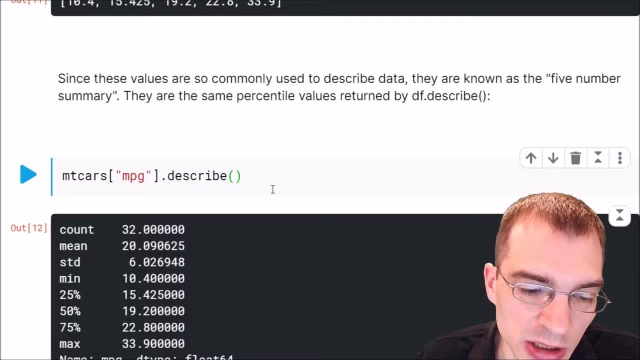 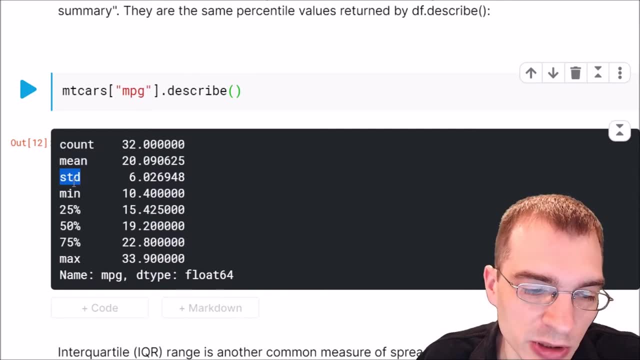 provide these five numbers as well as some other statistics like the median, So when we run that we can see the count median standard deviation, which is another measure of spread that we're going to look at in a second here. min the percentiles and the max Interquartile range, or 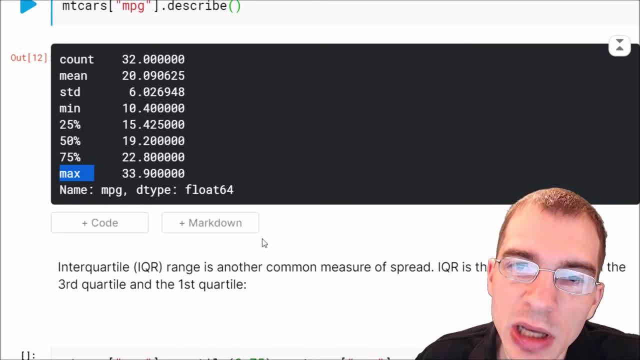 IQR is another common measure of quantile value. So we're going to run this and we're going to measure the quantile value. So we're going to take the quantile value and we're going to measure the spread. The interquartile range is the distance between the third and first quartile, So that 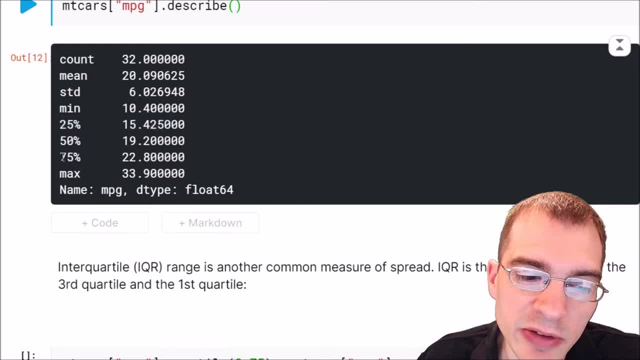 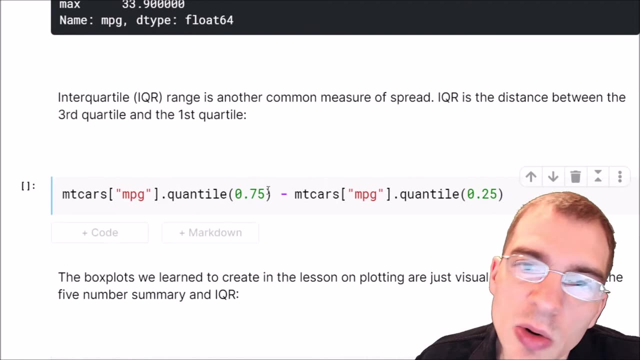 means between this 25 percent and 75 percent. 50 percent of the data is contained between these two quartiles and usually provides a pretty good bound for the bulk of the typical values of a distribution. To get the interquartile range we could just use our quantile function and subtract. 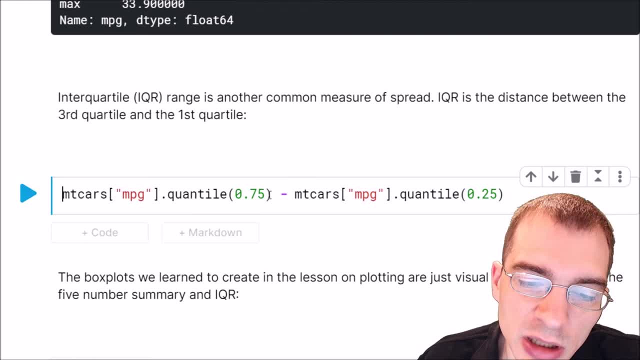 the first quartile, the 25th percentile and the rest of the quantile. So we're going to get the quantile from the 75th or third quartile. So in this case the interquartile range is about 7.3 miles. 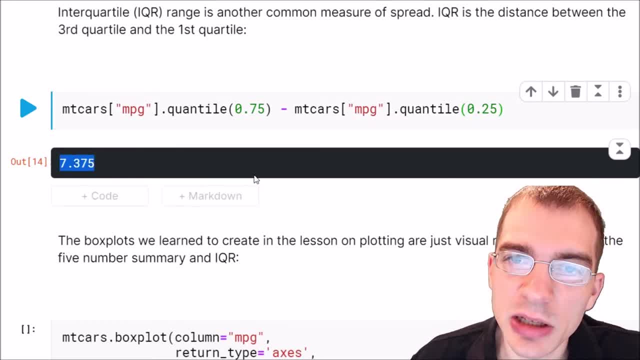 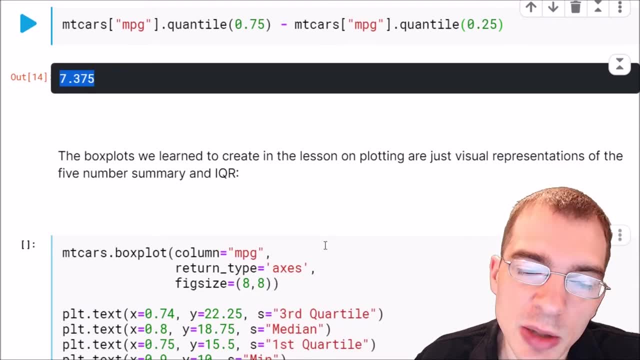 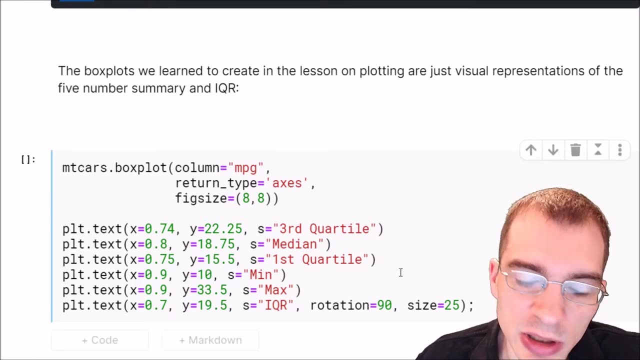 per gallon. The box plots we learned how to generate in the previous lesson on plotting in pandas is actually a visual representation of the five number summary and interquartile range. So here we're going to pull up a box plot and just explain where the five number summary and 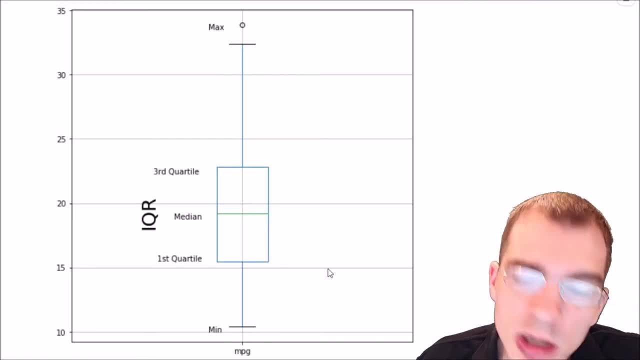 interquartile range appears. So this box plot, along with the text, kind of shows you the anatomy of a box plot and how the different key values match up with the plot. So the median is the green bar in the middle. The box here is the interquartile range with the first quartile or 25th percentile. 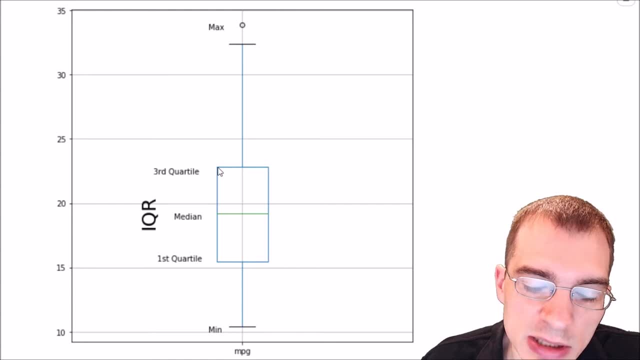 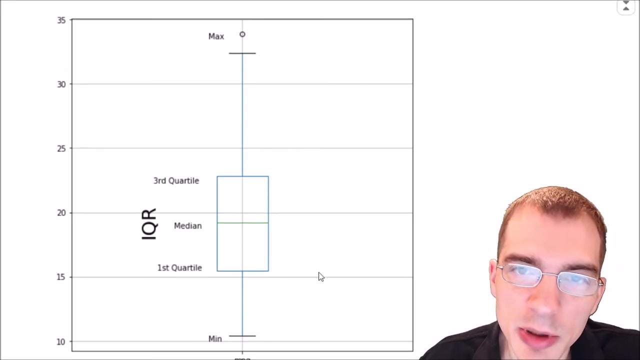 at the bottom and the third quartile or the 75th percentile at the top, And then the maximum value is the. whatever the highest value is, which in this case is this outlier circle, And the minimum value would just be where this black bar is Now. two other common measures of spread are variance. 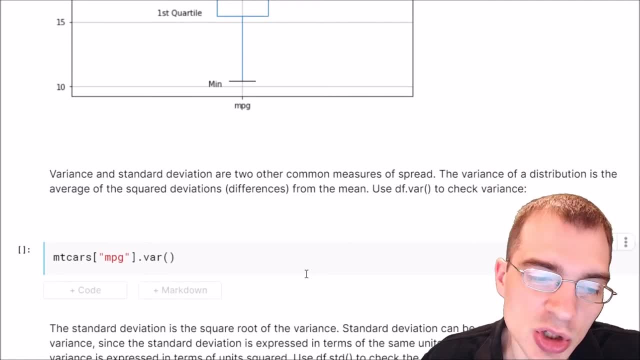 and standard deviation. The variance of a distribution is the average of the squared differences that values have from the mean. So basically, to find the variance, you first find the mean, Then you take that mean and for every value you subtract it from the mean, square it and 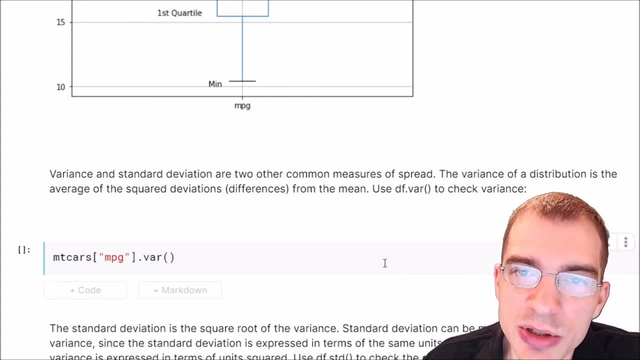 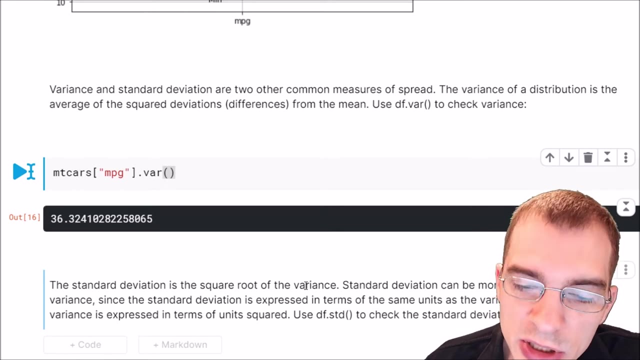 then you find the average of all those squared differences. To check the variance of a variable you can use the dot var function. So here we can take our mpg column and run dot var on it. That's showing us the variance is 36.. And the standard deviation of a distribution is the square root. 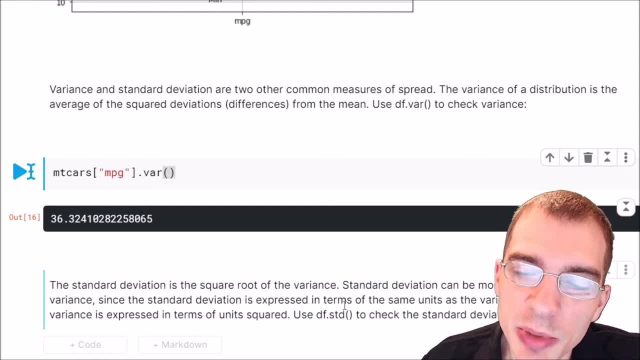 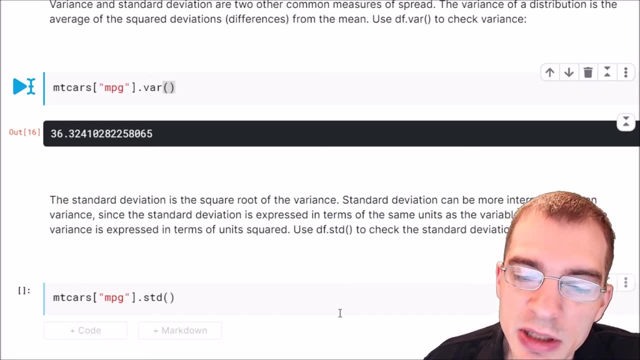 of the variance. Standard deviation can be a bit more interpretable than the variance, because standard deviation is expressed in terms of the variance of the variable. So if you're going to use the same units as the variable in question, whereas the variance is expressed in terms of, 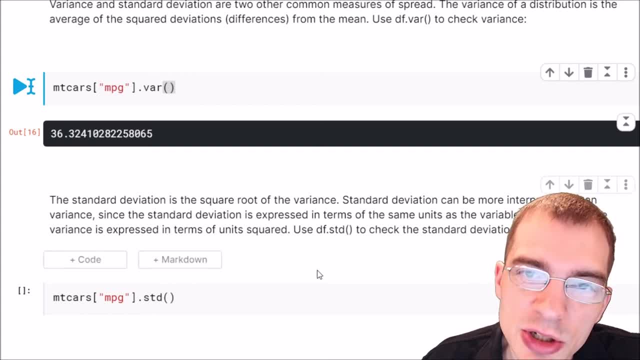 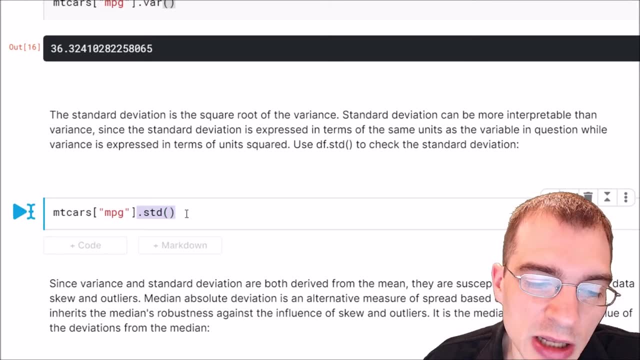 squared units, which is a bit harder to get a handle on. So to check the standard deviation you can use the dot std function. So we'll take the mpg column again and run standard deviation on it. So for this data set there is a standard deviation of about six miles per gallon. Now note that since 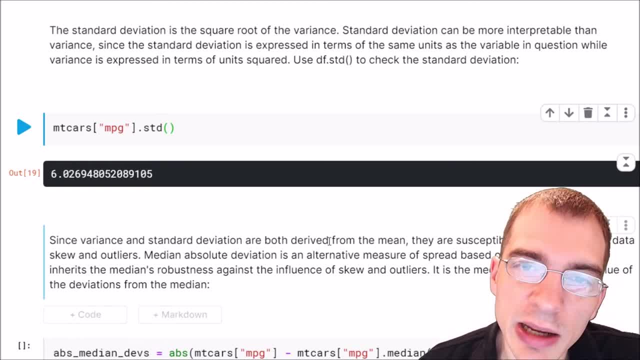 both variance and standard deviation are derived from the mean. they are susceptible to the influence of skew and outflow. So if you're going to use the standard deviation, function you, because the mean is susceptible to skew and outliers. Median absolute deviation is an. 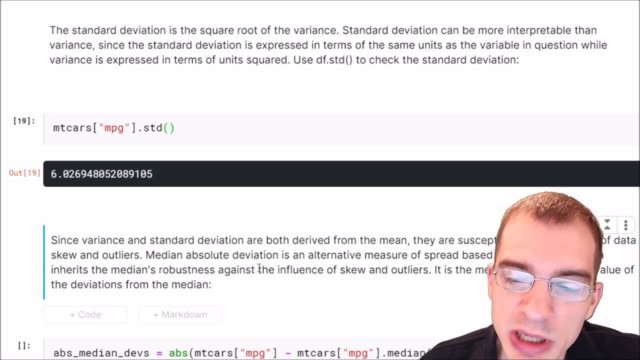 alternative measure of spread to the mean that is based on the median, which inherits some of the median's robustness against the influence of skew and outliers. The median absolute deviation is the median of the absolute deviations from the median value. So basically what that means. 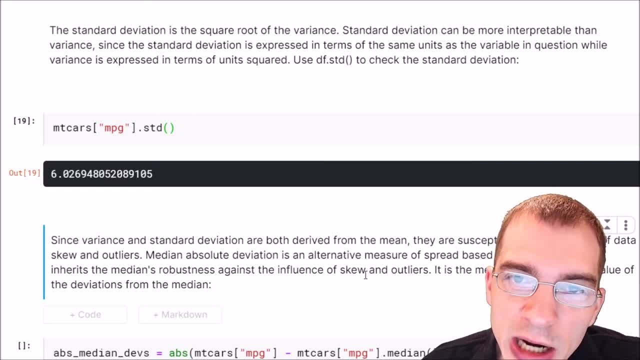 is you find the median of the data, you subtract all of the median writer value and you multi-duw料. You can find such data. So if you're going to use the standard deviation of about six miles per gallon, you can find. 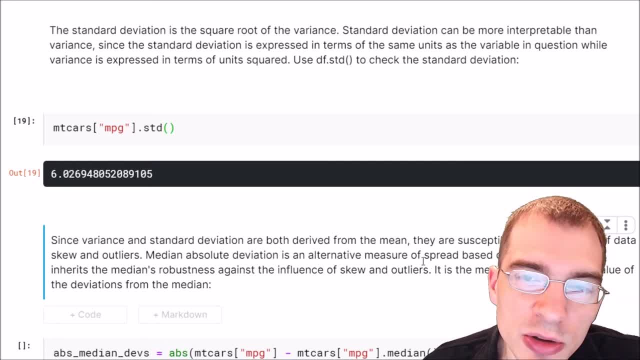 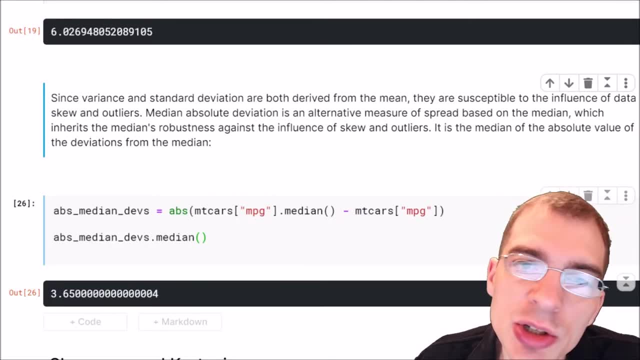 measure of spread to the mean. So this is an alternative measure of spread to the median value values. from the median you take the absolute value of all those differences and then you find the median of those differences. so to get the median absolute deviation we can start by taking 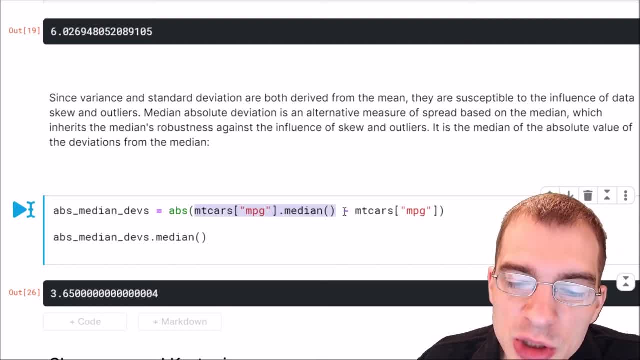 the median of our mpg column. we then subtract all of the mpg values in the column from that median. we'll take the absolute value of that whole quantity and save it, and this gives us all of our absolute deviations. then we just have to take the median of that. so we'll take our absolute. 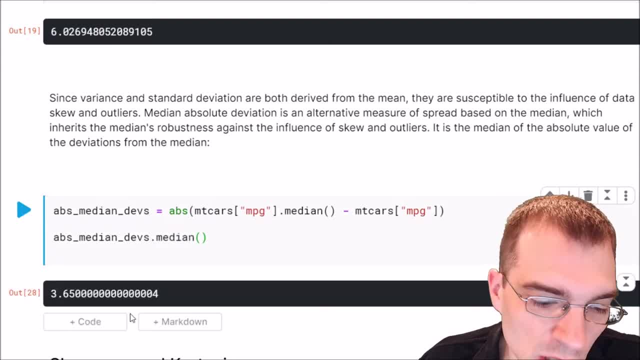 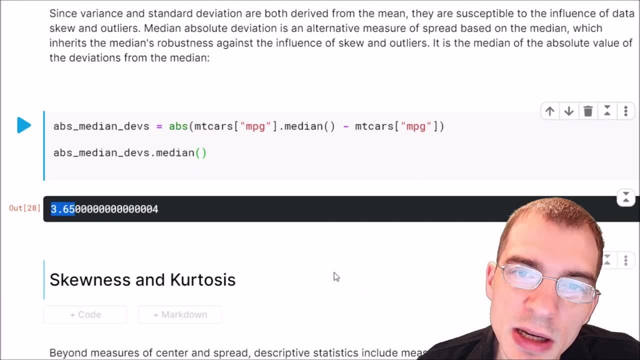 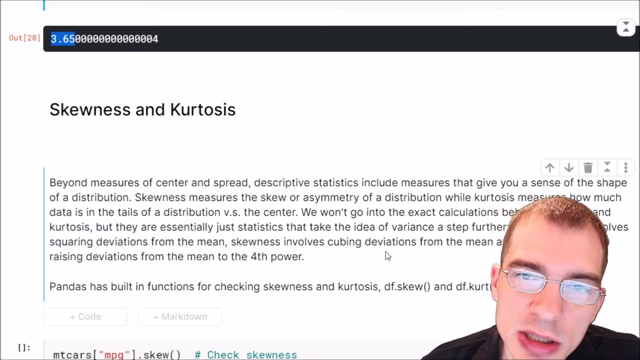 deviations run dot median on it and that gives us our median absolute deviation, in this case 3.65 miles per gallon, beyond measures of center and spread. there are some other statistics that give you a sense of the shape of a distribution. skewness is a statistic that measures the skew. 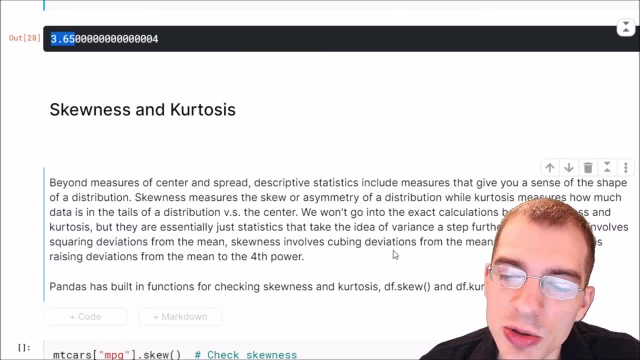 or asymmetry of a distribution, while kurtosis measures how much data is in the tails of the distribution versus the center. now we're not going to go into the exact calculations behind skewness and kurtosis in this video, but they're essentially statistics that take the idea of variance a step further, while variance involves squaring. 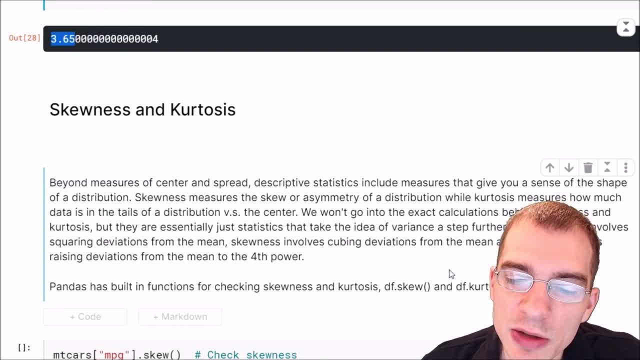 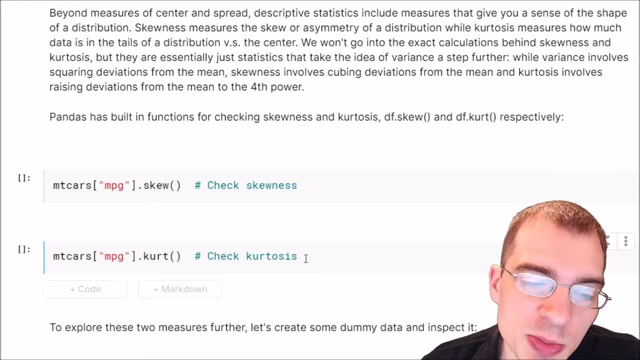 deviations from the mean. skewness involves cubing deviations and kurtosis involves raising those deviations to the fourth power. pandas has built-in functions for checking the median, so we can run a data frame that's skew and data frame that kurt respectively. so we can use those. 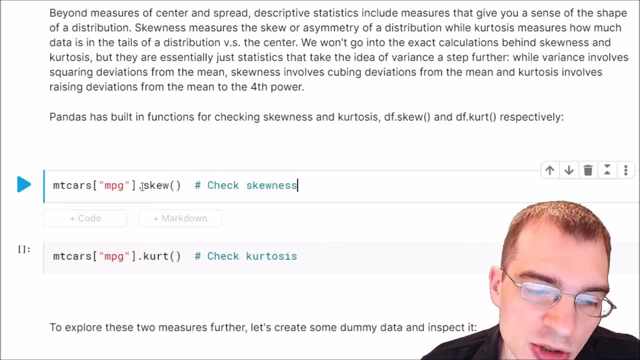 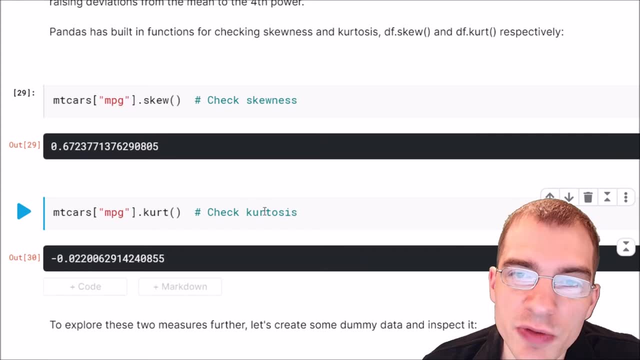 on the mpg column to check their statistics. so let's run dot skew on the mpg column to check its skewness and let's also run dot curt on it to check its kurtosis value. now these values we generated for skewness and kurtosis don't really mean a lot to us if we don't have any. 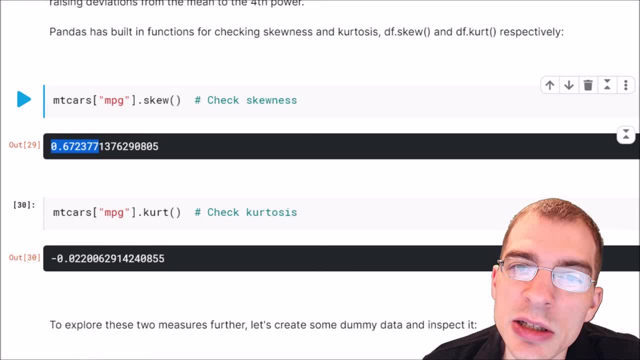 frame of reference for how much skewness this really is or how much kurtosis this is. So, to explore these two statistics a little bit further, let's generate some dummy data with different distributions and then rerun these functions on them to see how they differ. 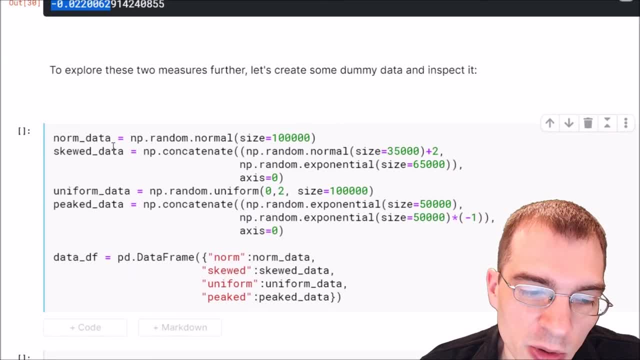 So we're going to generate four different distributions here. We're gonna make some normally distributed data, some skewed data, some uniformly distributed data and some peaked data, which is data with a pretty sharp spike in the middle. I'm going to run that to create our data. 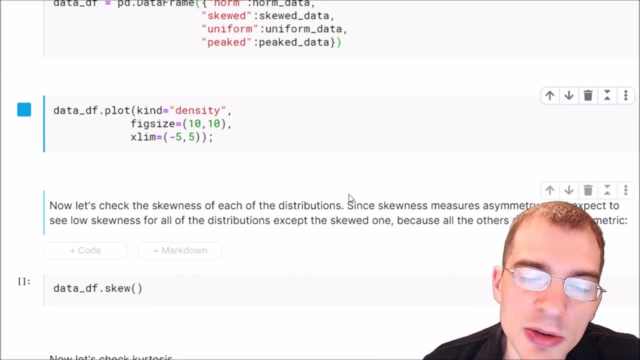 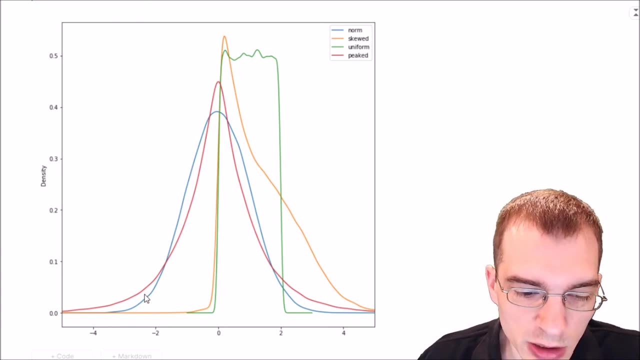 and then generate a plot of it so we can compare how the different distributions look. So in the resulting plot here we can see our four different distributions. The blue one is the normally distributed data. The red one is the peaked data which looks similar to the normal distribution. 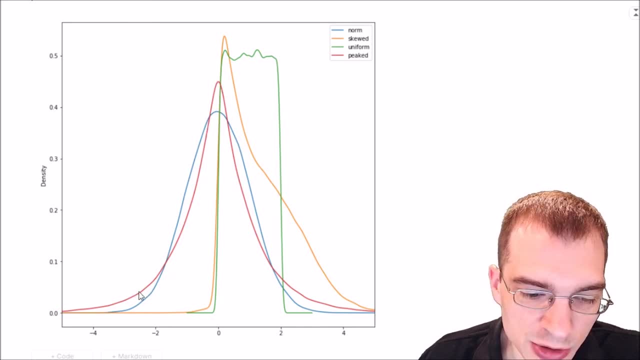 It just has a sharper spike in the middle and tails that are longer. The skewed data is the orange distribution, which has a big spike and then goes off more to the right, And then the uniform distribution. the green one just samples values evenly from a given range. 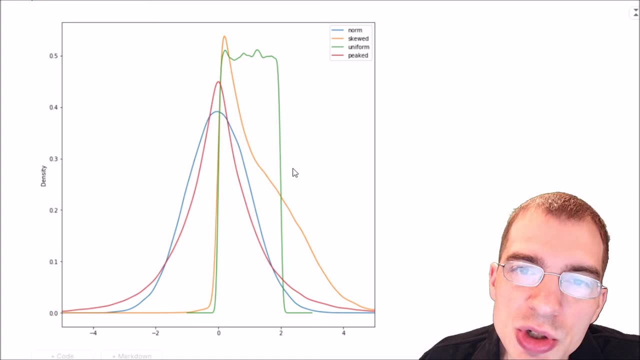 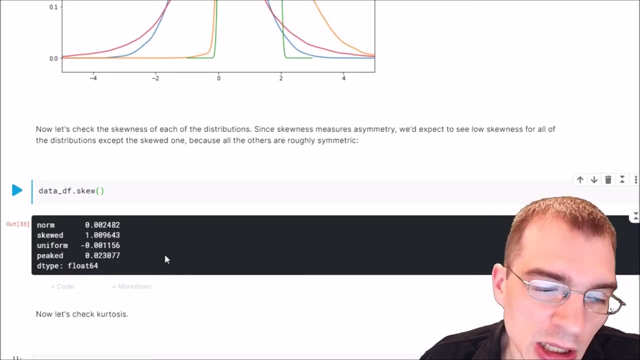 So let's take these four different distributions and run skew and kurtosis on them to see how the values differ. So we'll start by running skew on our data frame here And we can see that for the normally distributed data the skew is almost zero. 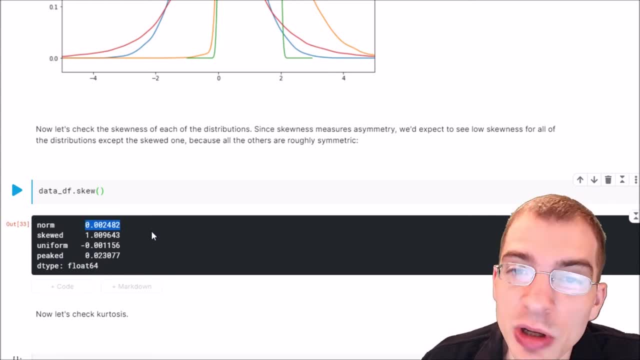 That's because a true normal distribution doesn't have any skew at all. Now the heavily skewed data has a skewness of around one. The uniform distribution is also very close to zero because that has no skewness to it either. and again, the peak distribution has almost no skewness because 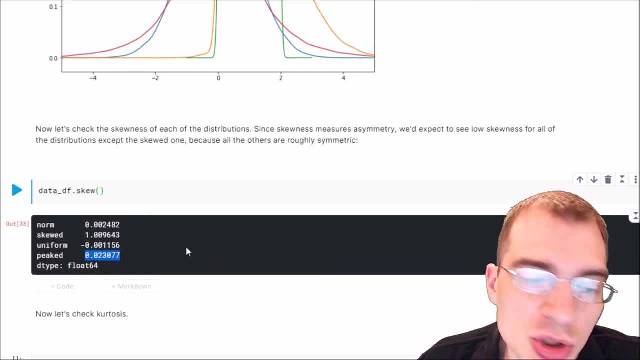 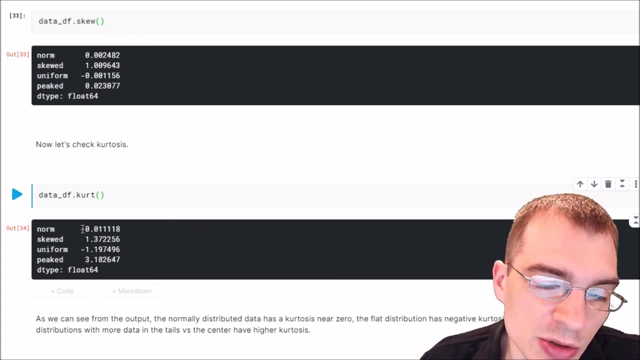 it is symmetrical, even though it's not normal. now let's run the kurtosis on our different distributions. so the normally distributed data has a kurtosis value near zero. the skewed data has a kurtosis of 1.37. that's probably because with the skewed distribution you have a bit more.